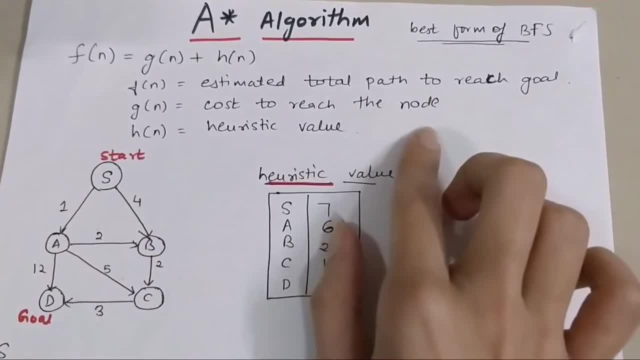 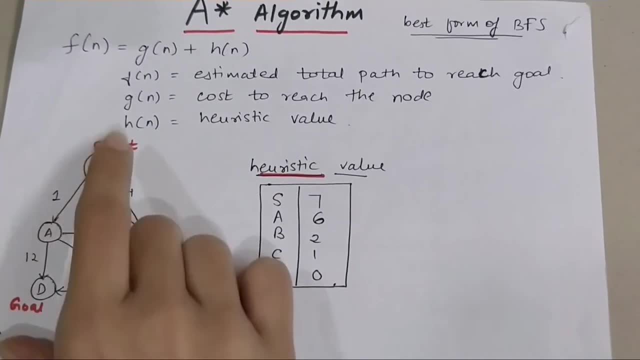 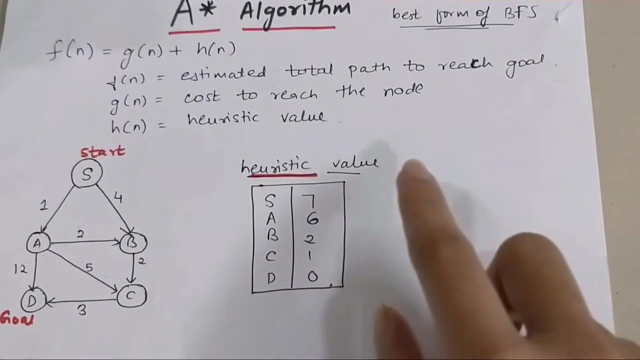 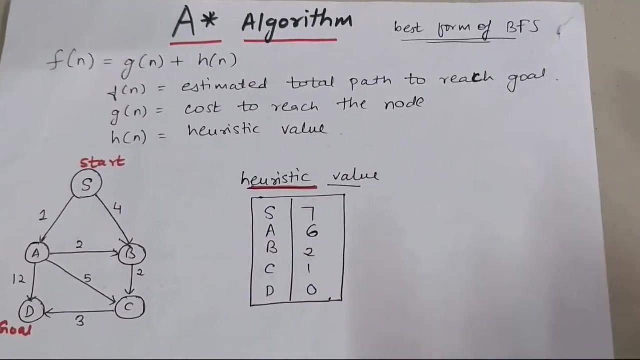 f of n for every particular node. What is g of n? Cost to reach the node? So basically, s to a. So what will be g of n? 1, the cost to reach that particular node, s to d, will be 1 plus 12, which is 13.. Okay, that is g of n. h of n is heuristic value. Heuristic values will be given in the question itself And I am not going to go into theory much in this video right now. If you want a video on heuristic value, let me know in the comment section. I will make one on it. 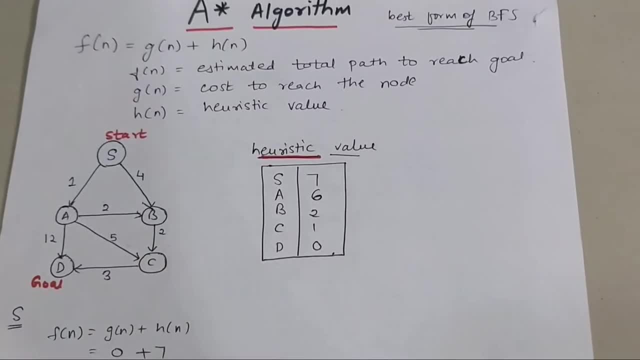 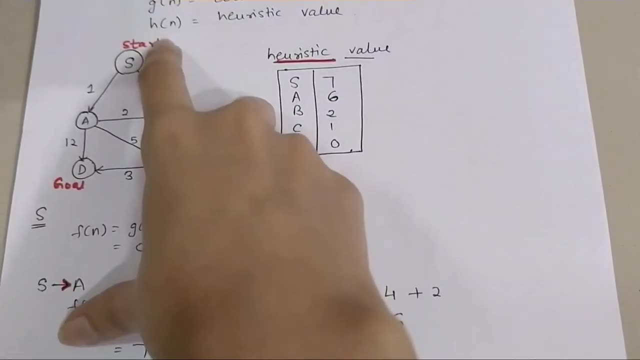 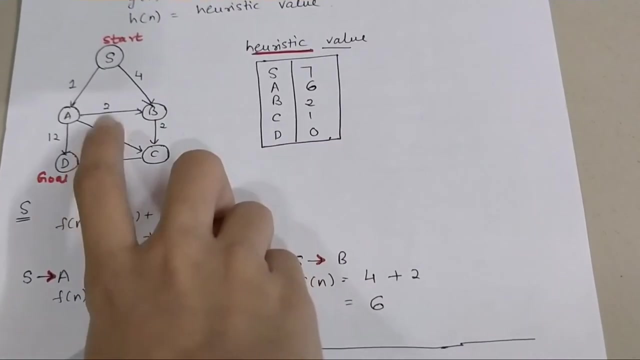 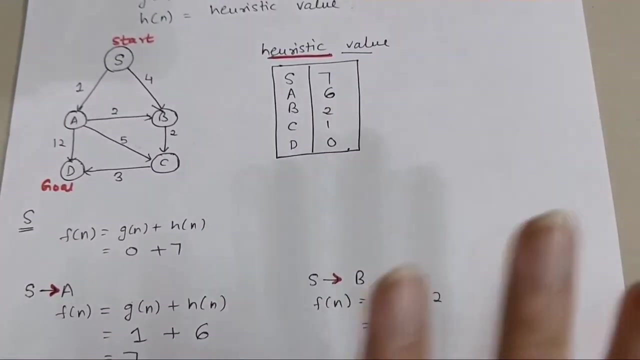 For now. for now, let's see an example. Okay, So this is the example. These are nodes s, a, b, c and d. s is the start node and d is the goal node. Basically, from s we have to reach d And which path we have to use. that A star algorithm will tell us. Okay, And these are the heuristic values of every particular node, every node, Okay, So let's start solving this up. First we're going to take the node s. 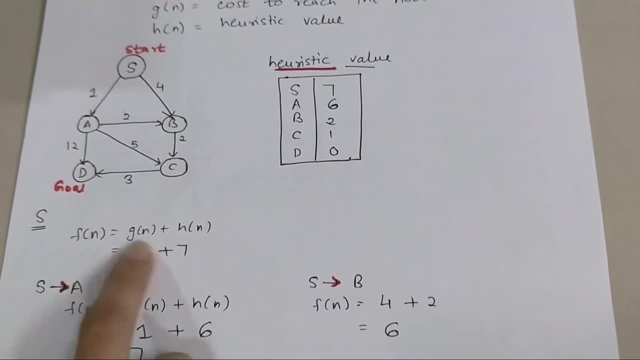 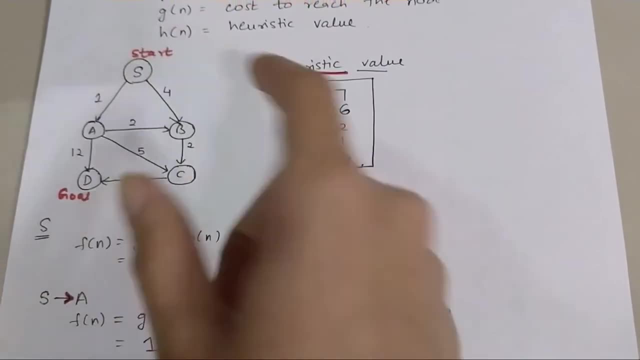 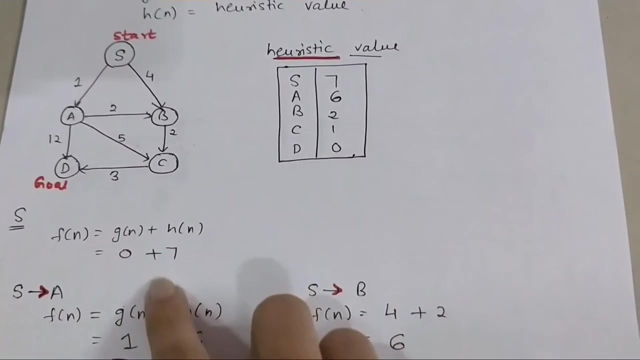 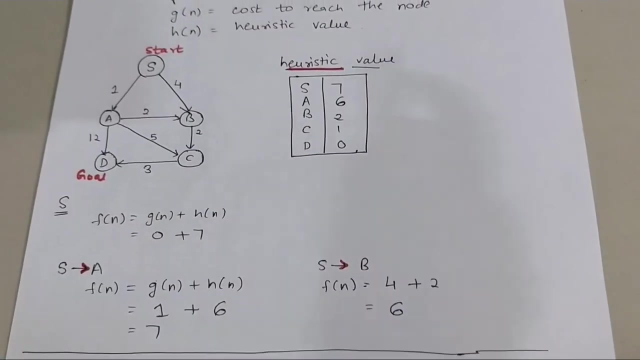 And we're going to calculate f of n for s. Now, for s, f of n is equal to g of n plus h of n. Now g of n is the distance to reach that particular node. For s to reach, s will take how much? How much cost? 0, because it is going to reach to itself only. That is going to be 0. And h of n is going to be the heuristic value. So heuristic value of s is 7.. So 0 plus 7, which is equal to 7.. Now, from s, we have two nodes. Okay, 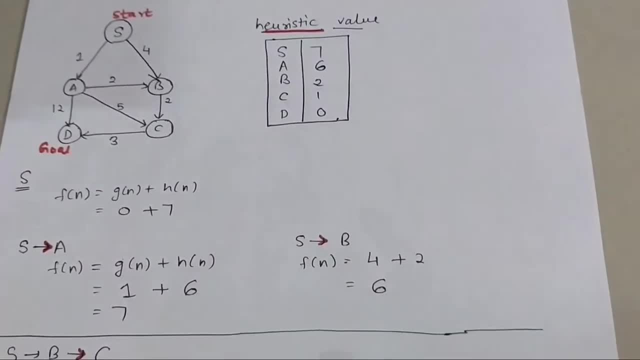 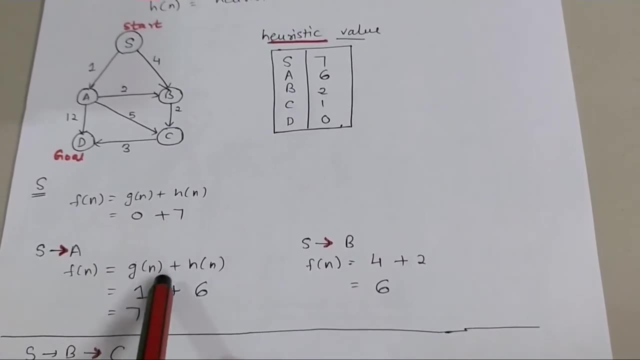 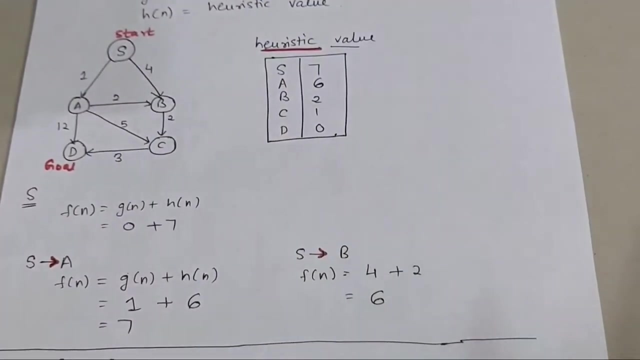 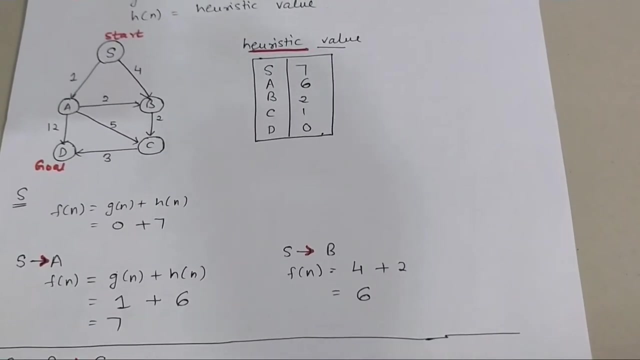 And we can go to A, either to A or to B. So we have to calculate f of n for both, for s to A and for s to B, both. So for s to A, f of n is going to be g of n plus h of n. g of n is the cost to reach that particular node. So the cost to reach A from s will be how much? 1.. Hence 1 is written off here. h of n is going to be the heuristic value And if you want to calculate heuristic value it is going to be of the node we want to reach. So basically s and b. 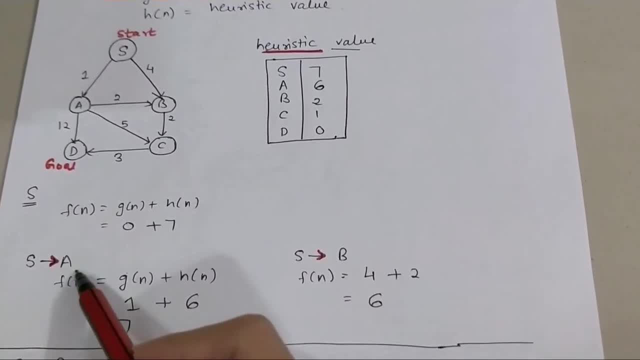 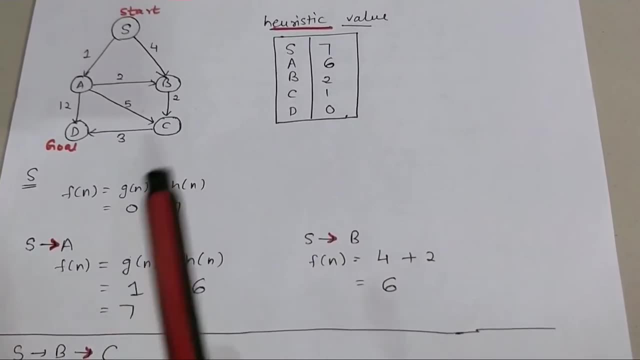 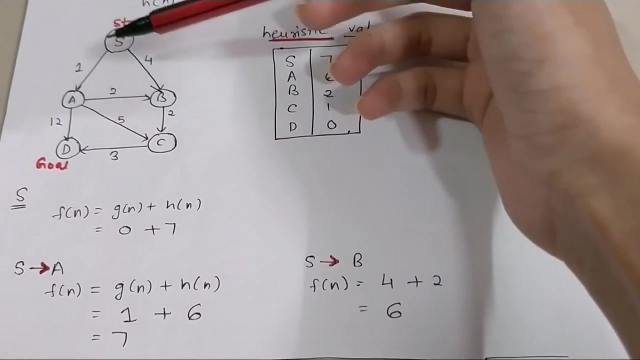 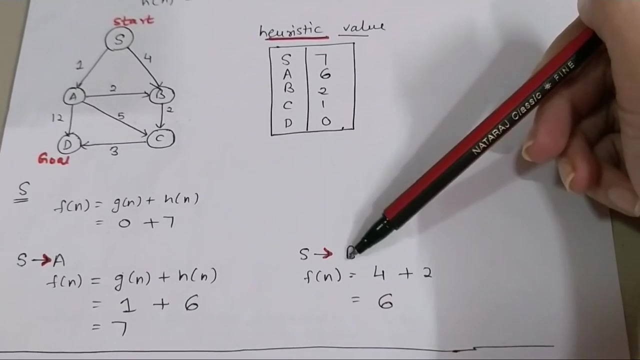 We have to reach which node, A. So we are going to take the heuristic value of A, which is 6.. So 1 plus 6 is 7.. This is our f of n for s to A. Now for s to B, f of n is going to be first of all g of n, that is, distance from s to B, which is 4.. And heuristic value of B, because we have to reach B. Okay, Whichever node we want to reach, the heuristic value of that particular node is to be taken. 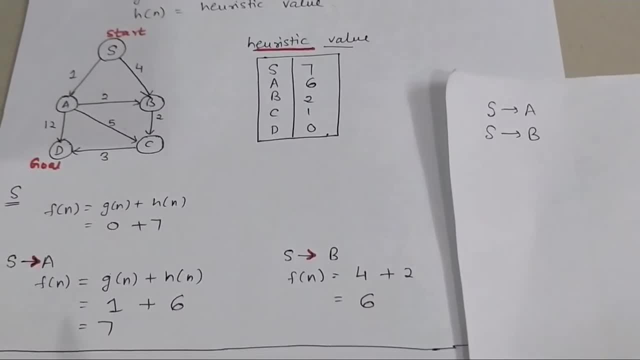 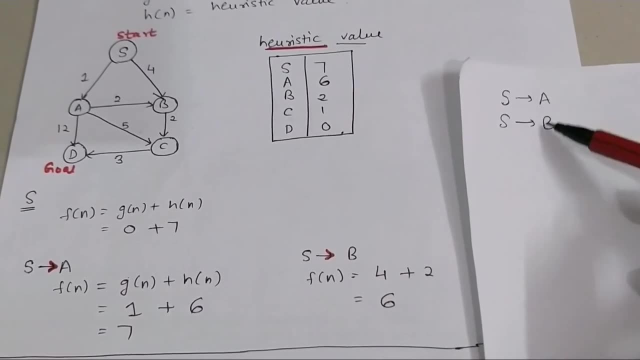 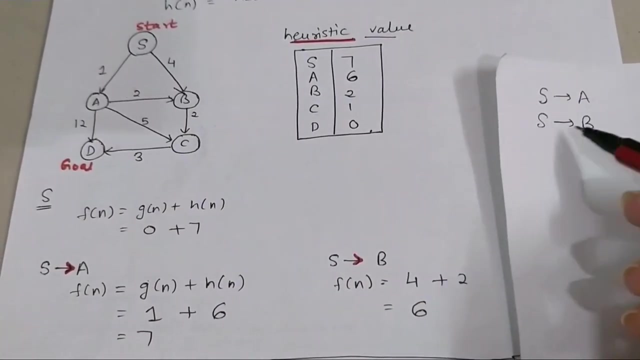 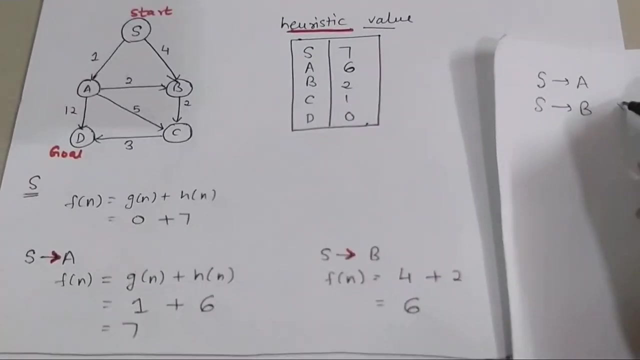 So heuristic value of B is 2.. So this is f of n for both of them. Now we have to maintain all of these paths at one section of the paper or at one place. So I have written s of A over here, s of B over here, which is least 6th one. So I am going to use 6th one, So I am going to put a cross over here, And next thing I am going to do is calculate from s to B. Okay, 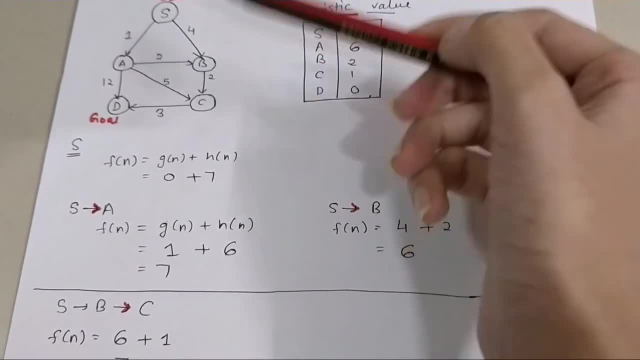 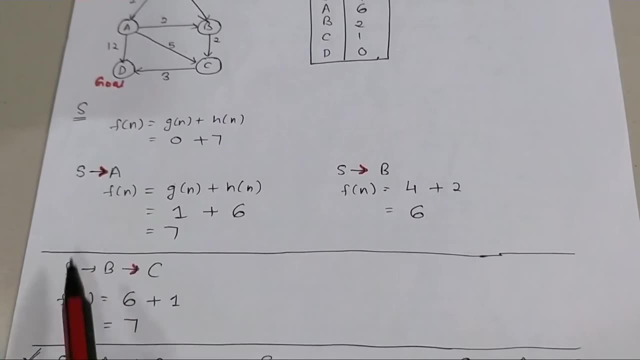 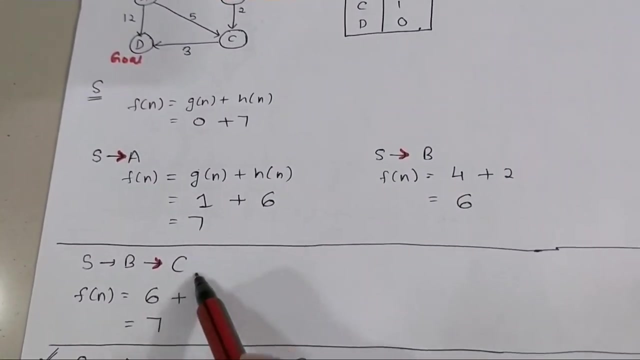 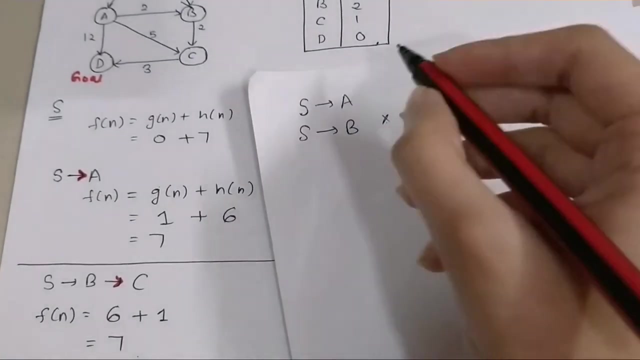 Now, next thing, which node can I reach from s to B, s to B to C? So I am going to write s to B to C. So f of n is going to be g of n. that is the distance we reach C from s. So which is going to be s to B is 4, B to C is 2, that is 6.. Hence 6.. Plus heuristic value of C, which is 1.. So 6 plus 1 is 7.. Okay, Then again, I am going to note it down on a piece of paper. So s to B to C. 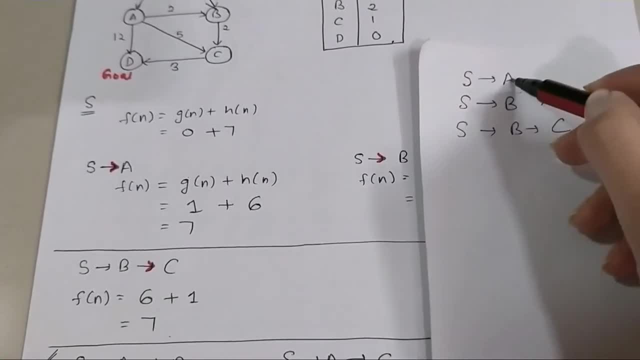 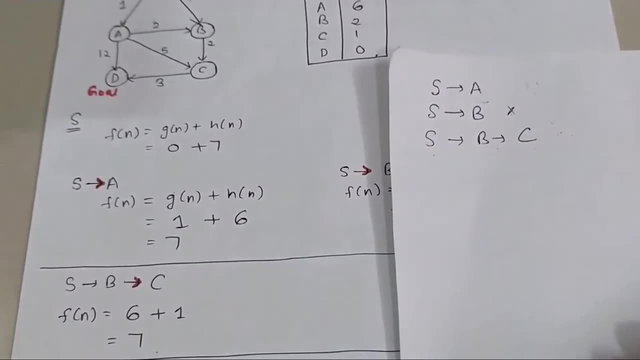 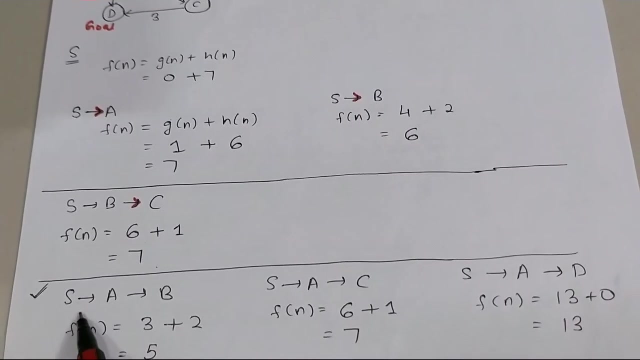 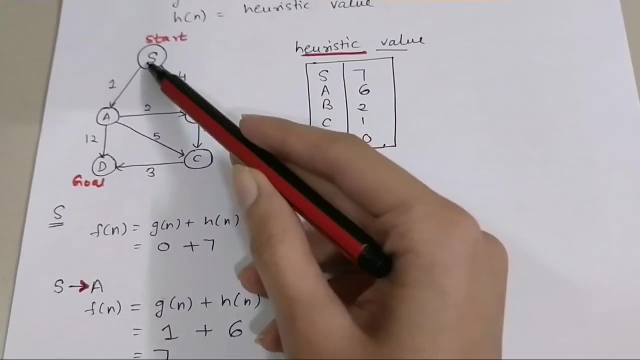 Okay Now, what is the value of g of n? What is the value of s to A? 7. What is the value of s to B to C? 7. Both are equal, Hence we have to check for both of them. Okay, So first I am going to check for s to A, Now for s to A, Now for s to A. I have three ways I can reach. I mean I can go ahead. So one is s to A to B, next is s to A to C, third is s to A to D. So I am going to calculate. 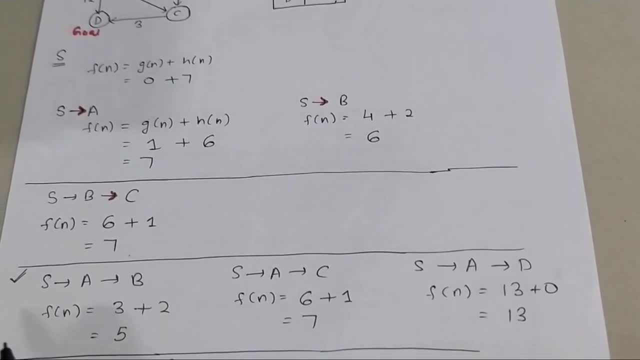 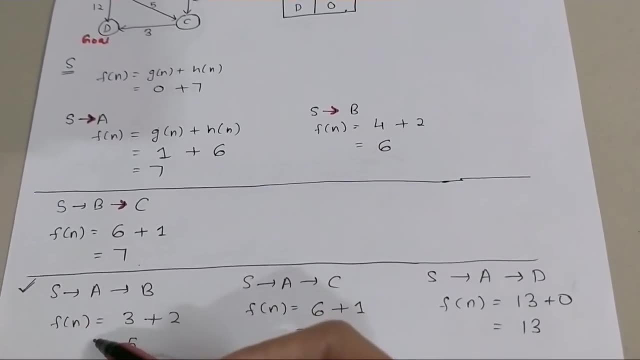 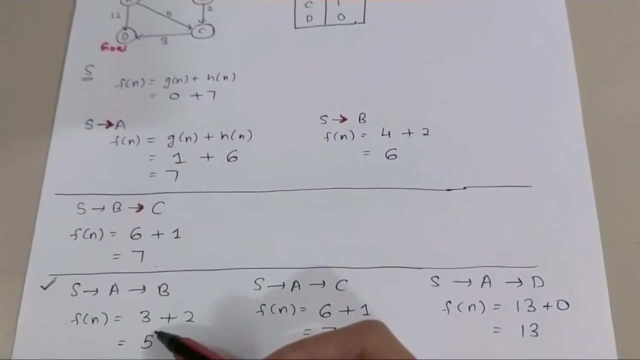 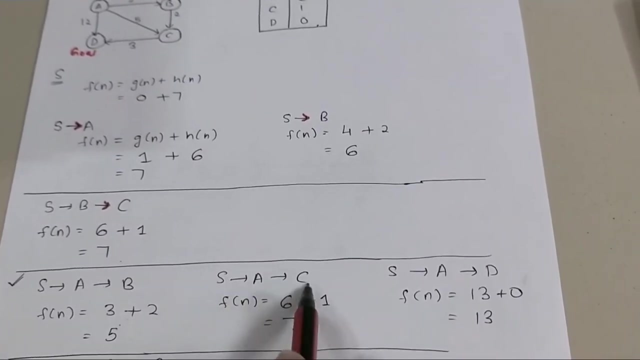 s to A to B, s to A to C, s to A to D. So f of n is going to be g of n plus h of n for the three of them. Okay, So let's calculate. So f of n is going to be distance we reach, s to A to B, which is going to be 3. Plus the heuristic value of B, which is 2.. Hence 5.. And similarly, I am going to calculate for s to A to C, s to A to D. 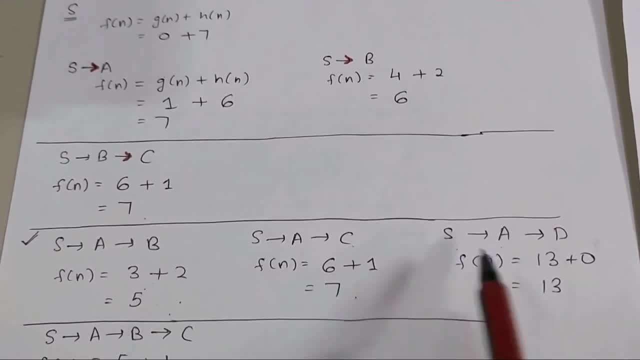 Okay, These are the values I have got for them: s to A to B, s to A to C, s to A to D. Now again, I am going to write it on a piece of paper. I mean on the same list. I am going. 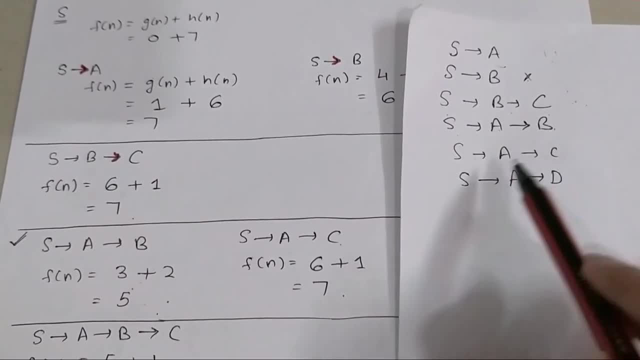 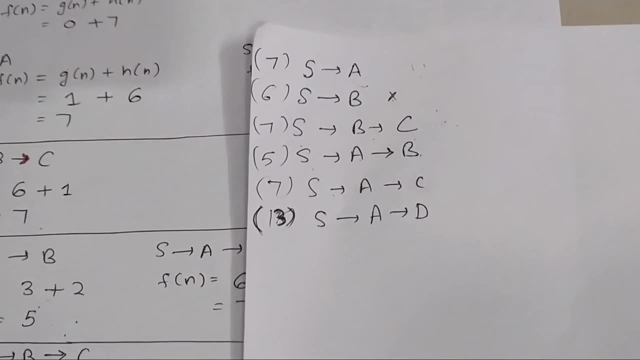 to add it to that. I am going to add it there. s to A to B, s to A to C, s to A to D. Now for which f of n is the least? Okay, Now again, I have added all these. Now, once I have put. 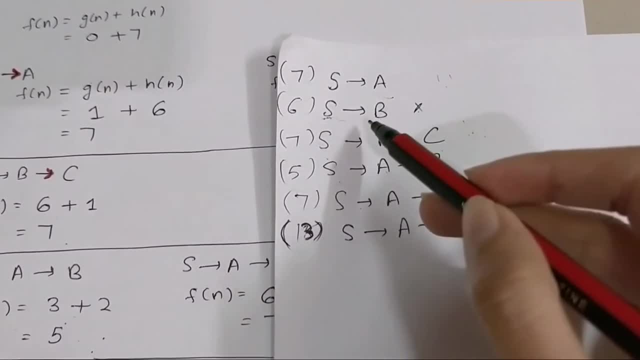 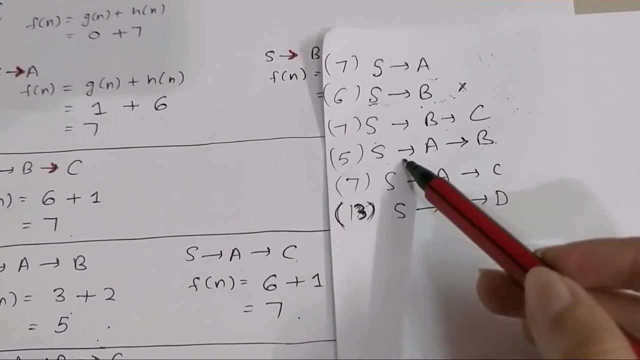 a cross on it, it means I have used this path. Hence I am not going to use it again Now I am going to use it again Now. in the rest of the paths, which is the last path, I am going to use the least value. This one s to A to B, because the value is 5.. Hence I 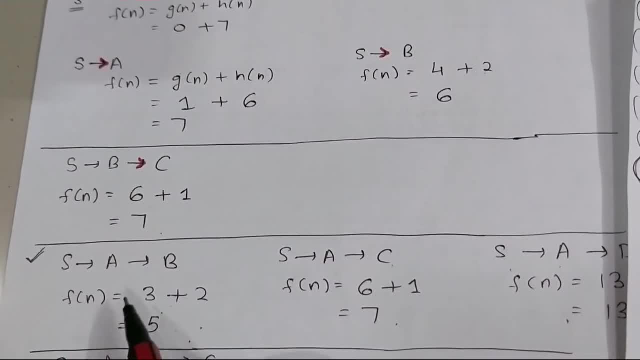 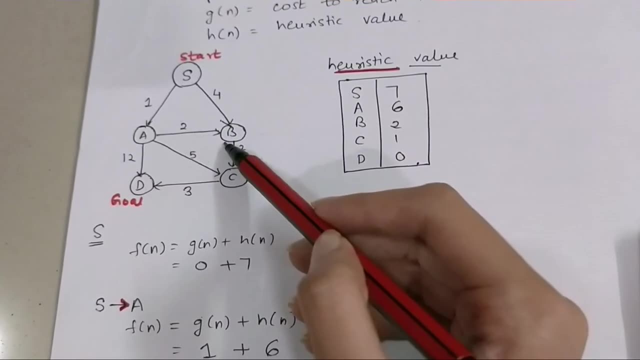 am going to go ahead from here, So I am going to choose the path s to A to B. Okay, Now s to A to B. what is the next node? c? Hence, I am going to take s to A to B, to C Again. 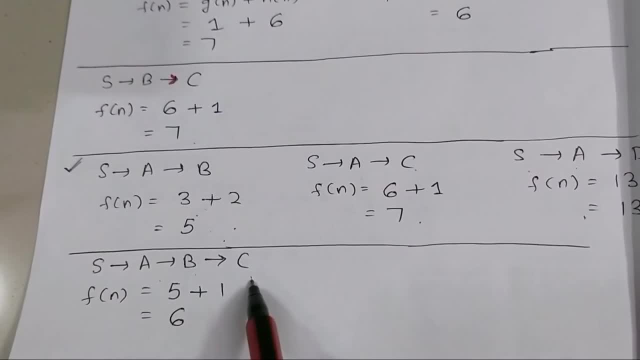 I am going to calculate f of n, Which is g of n plus h of n. Now what is going to be the g of n for s to A to B to C? Distance from s to A to B to c. This is the distance, distance. between the brackets which I have written here. distance between the brackets To which I am going to repeat it: dn 1 plus h. Now I am going to take the distance from b and part a, dotted by dn minus a. Again, I am going to take the path which I have written here: the guidance. 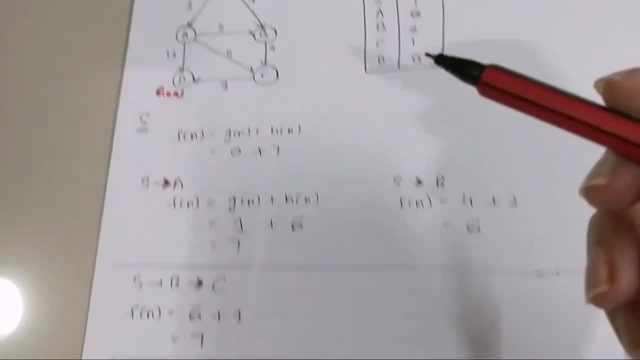 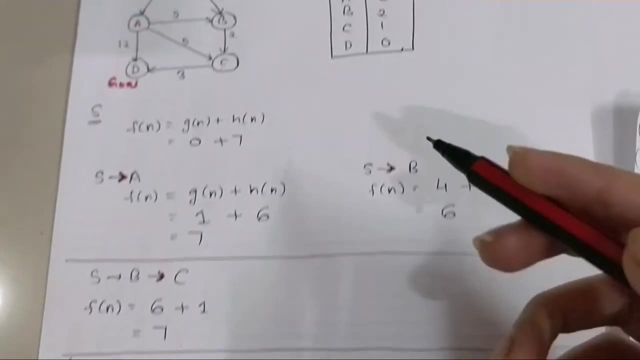 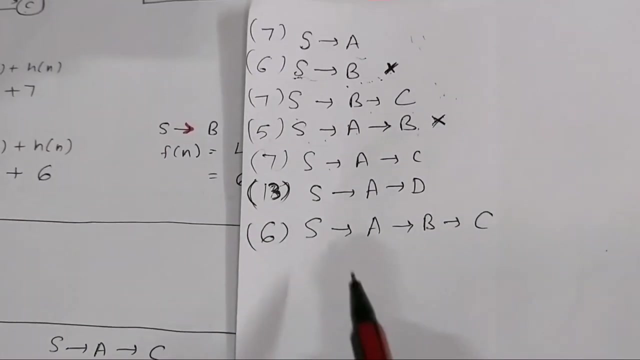 c, which is 2 plus 1, 3 plus 2, which is 5, 5 plus heuristic value of which node, the node we want to reach, which is c. heuristic value of c is 1, hence 5 plus 1, which is 6. again, i'm going to add: 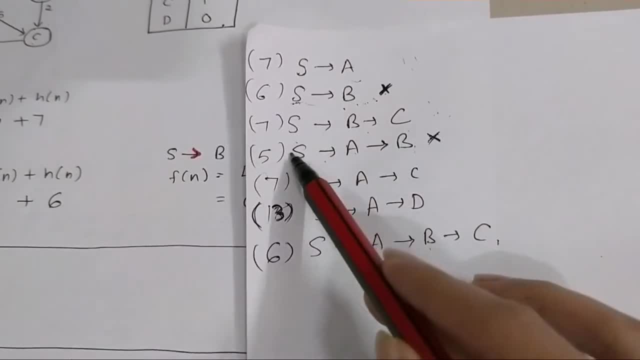 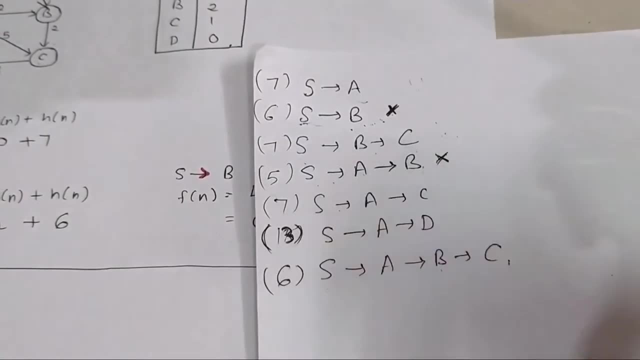 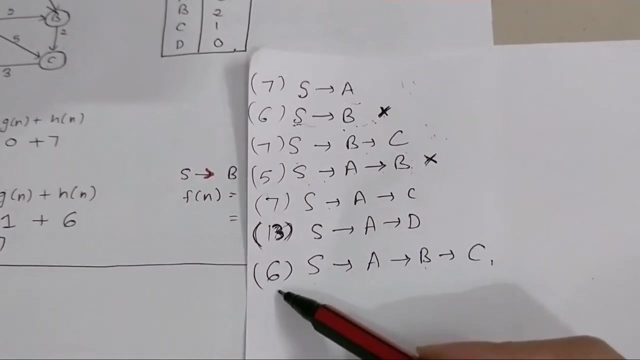 that in this particular list- and i'm going to put a cross over here because i have used this particular path- okay, now, s to a to b to c. now, which one is the least amongst all of them, except the cross ones? okay, because i have used them: 7, 7, 7, 13, 16, 6, so this is the least one. so i'm going to. 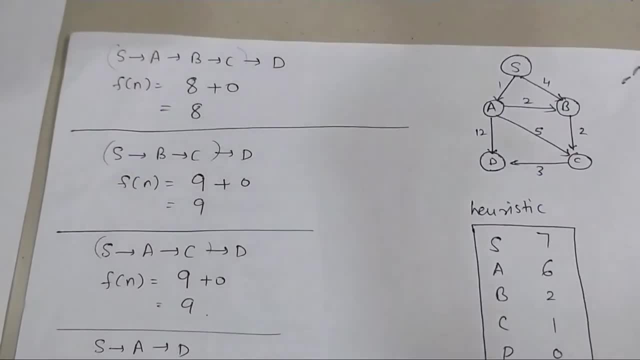 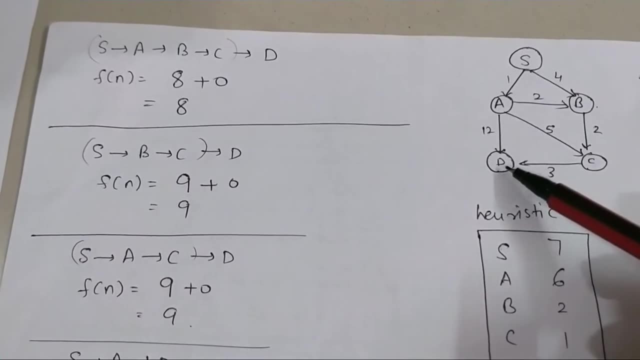 use this path. okay, now i am going to use s to a to b to c. now, for from your, which is the next node, d and d is our gold node. so s to a to b to c to d. now i have to calculate f of n, which is which. 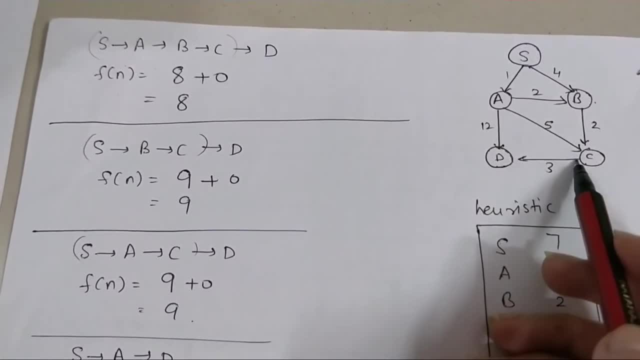 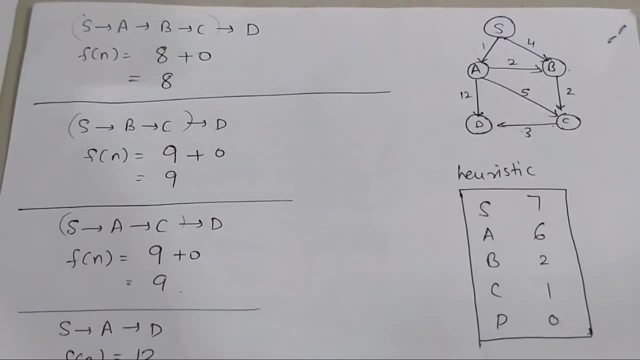 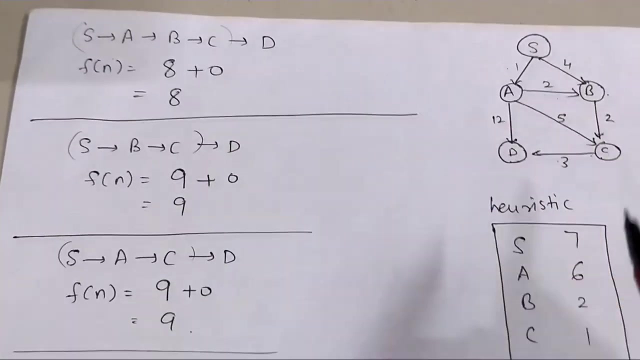 is going to be the distance from s to a to b to c. what is that? 8, 1 plus 2 plus 2, which is 5, 5 plus 3, 8 and 0 is the heuristic value, because the heuristic value for d is 0, so f of n for this particular. 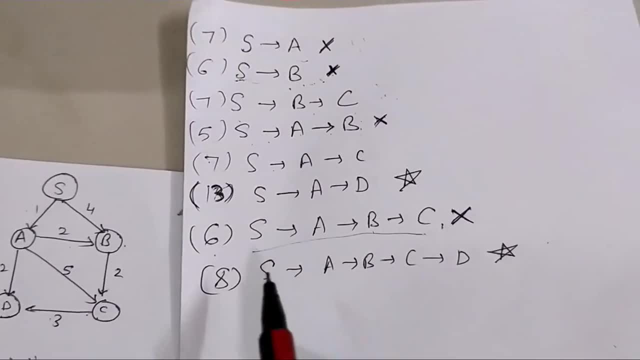 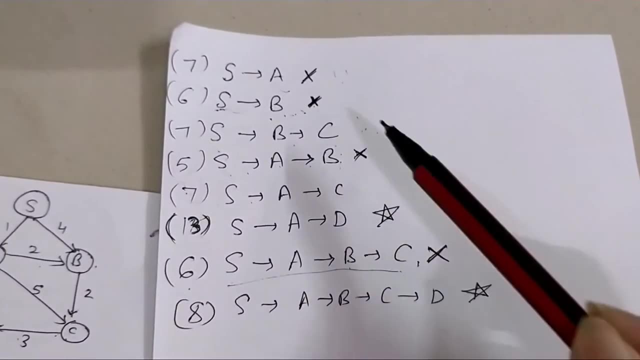 path is going to be 8, and then i'm going to add it to the list. okay, s to a, to b, to c, to d, and the value is 8. now, these are the crossed ones which are already used, so i am not going to consider them. 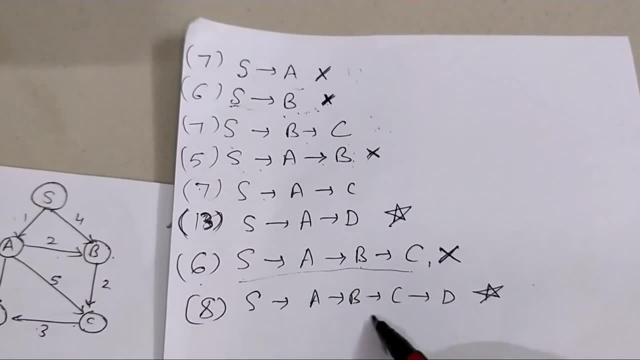 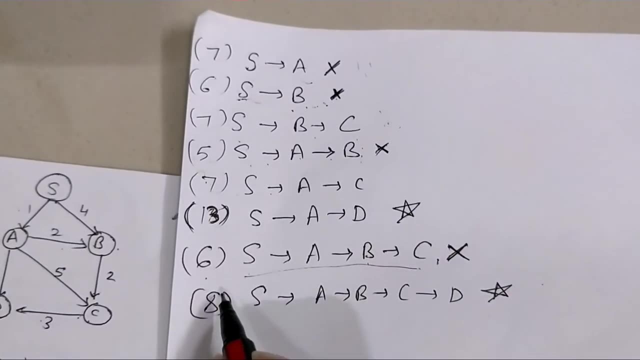 and also i'm not going to consider this one- s to a to d and s to a to b to c to d. why? because they have already reached their gold node. they have already reached the gold node, so now the value over here is 8. now i have to consider this, this and 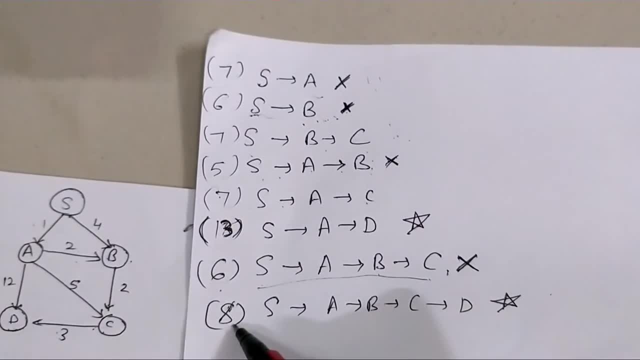 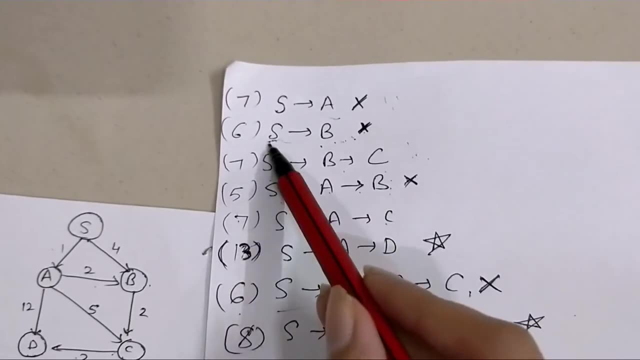 this and this and this one, because this is 8, the least one. okay, till now 8 is the least one, but as we see, s to b to c and s to a to c, have a. uh, have the cost as 7. sorry, have f of n and f of n. 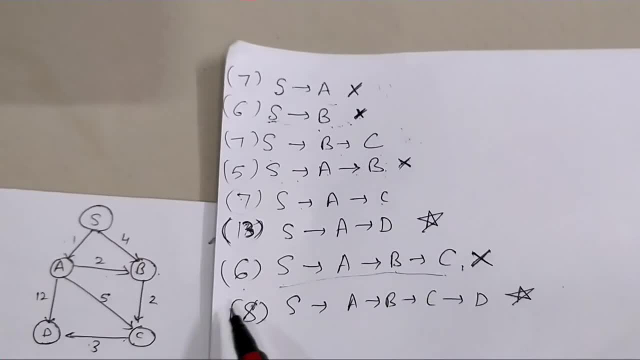 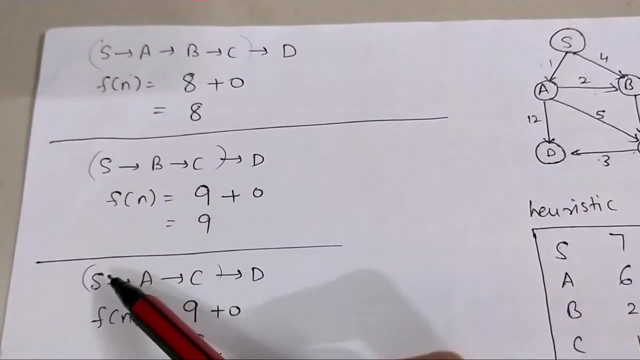 as 7, which is less than 8.. hence i have to also go through these two paths, so s to b to c and s to a to c, and from s to b to c to d, hence this one, and i'm going to calculate f of. 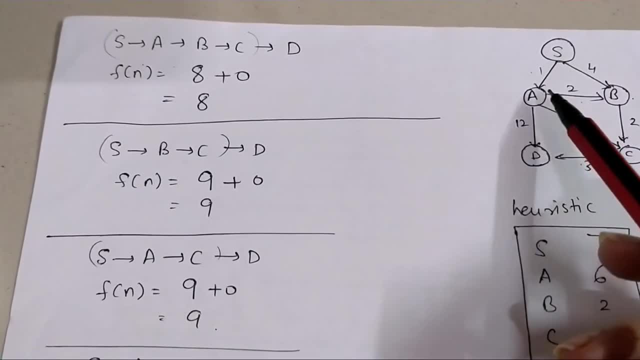 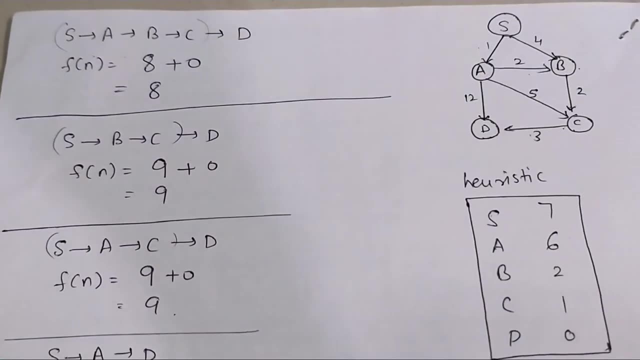 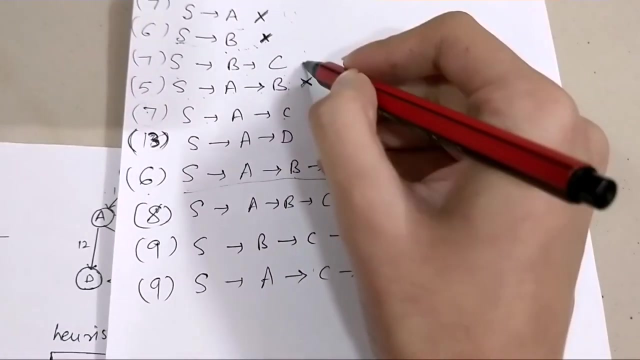 n, which is going to be 9, and similarly, s to a, to c, to d and f of n is going to be 9.. so these are the f of n's and then i'm going to add them to the list. okay, and i added them to the list, as you can see. so, uh, and, and these two are also used.